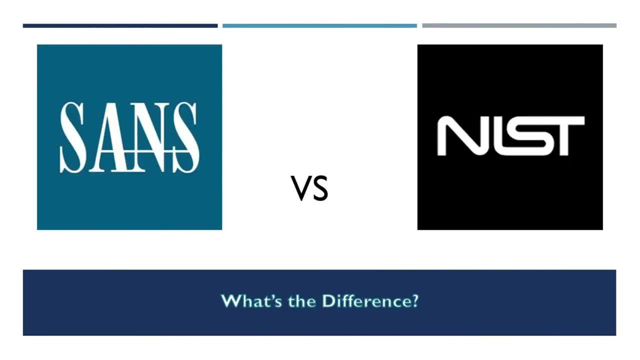 server to go down, which would affect the availability. So what is an Incident Response Lifecycle in cybersecurity? There are two main frameworks, one from SANS and one from NIST. The Incident Response Lifecycle is a set of steps and phases of an incident response plan, and an Incident Response Plan is a document that contains 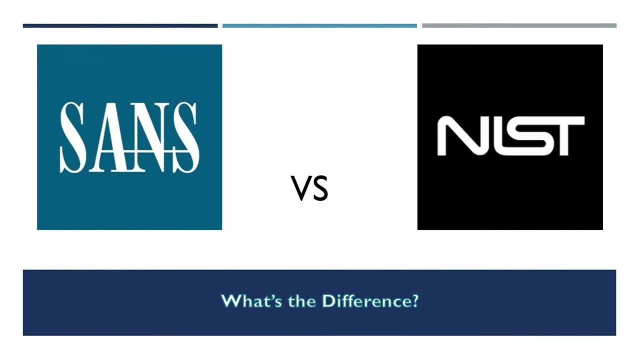 a set of instructions for a business during a cybersecurity incident. These instructions follow a specific set of steps, but the actual contents are going to be specific to that business. The document is designed to be a guide for a company from the very beginning, before the incident even occurred, all the way to the last phase of finding out how the 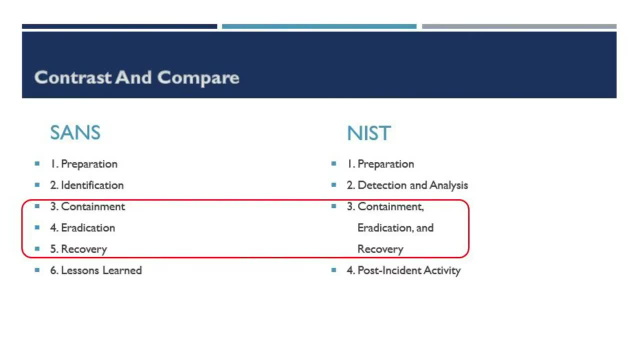 incident happened and how to prevent it in the future. Let's briefly contrast and compare the differences between the SANS and NIST frameworks. They're very similar and only go a little bit further than the SANS and NIST frameworks. They're only grouped and worded differently. It's good to know how to organize both, because 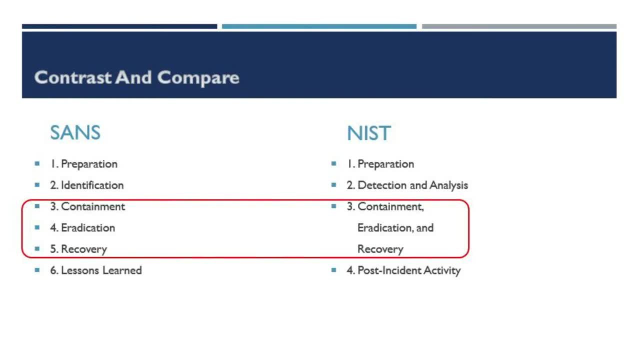 a future employer could request or require you to use either or. As you can see, SANS defines phase two as identification, but NIST calls it detection. and analysis, Containment eradication and recovery are all bundled into one for the NIST lifecycle. Finally, post-incident response falls into the same category as lessons learned. 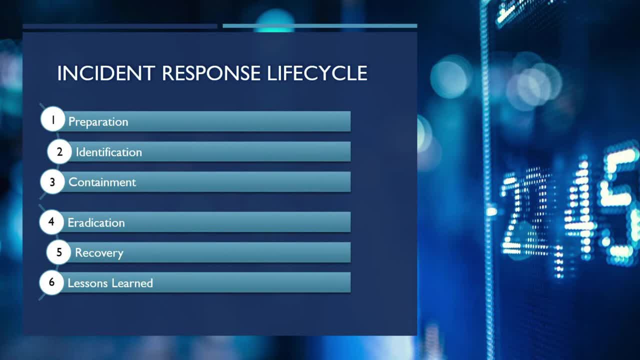 We'll define these more in just a moment. For this video, we're going to be doing it in the form of the SANS lifecycle and go through each of the six steps individually, and hopefully this makes things easier to understand. Step one is preparation. The first step is talking about developing the incident response. 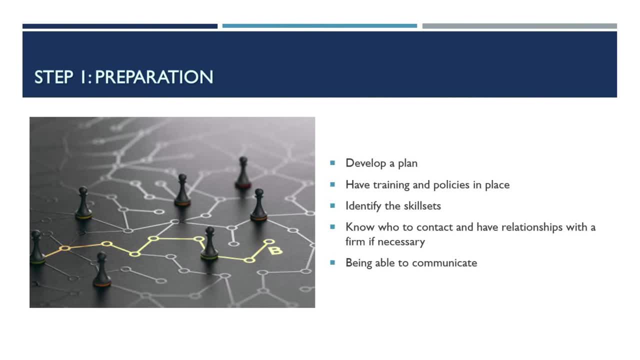 plan itself. The worst thing would be trying to figure out what to do while an attack is in progress, and that's never the time to figure out what to do while the incident occurs. It's much better to have something set up and organized. The organization includes things. 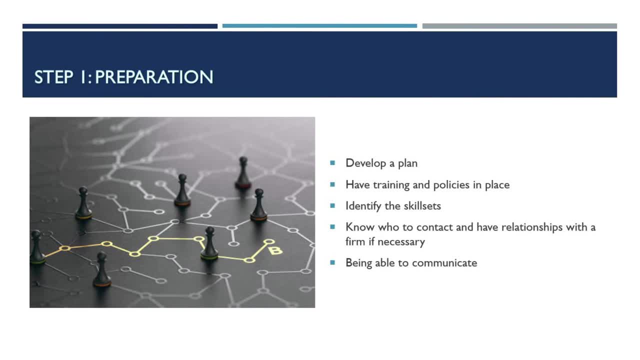 like getting your people ready and trained, identifying skill sets and having the procedures and policies in place, along with having the right tools or knowing where to get them. Some companies aren't equipped to handle the full-fledged cybersecurity incidents, so they may have 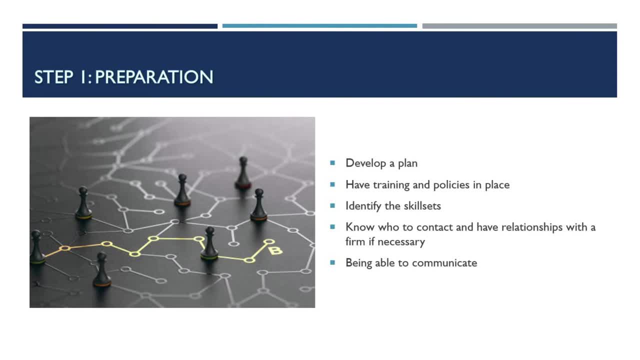 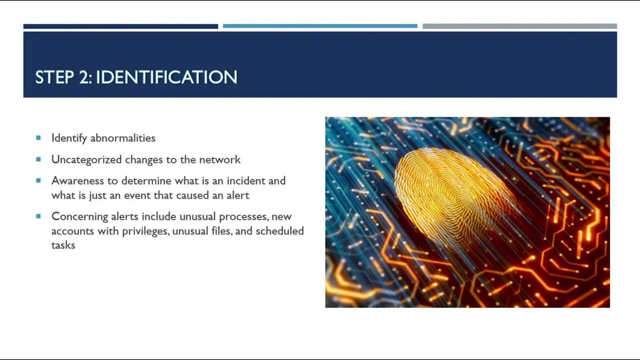 a firm to help. It's vital to have a relationship and proper communication plan with the selected firm instead of scrambling once that time comes. Step two is identification. This is the step where you would try and identify any abnormalities or unrecognized changes within the network. This step relies heavily on awareness and 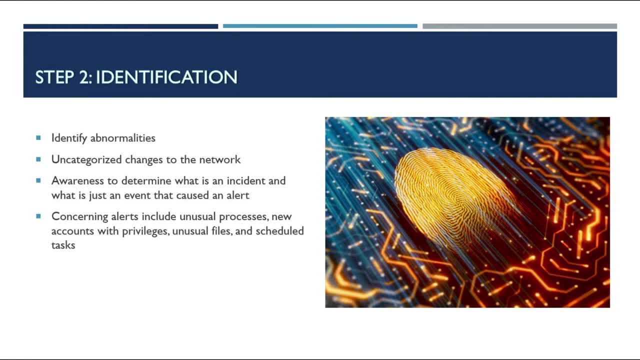 having the ability to identify whether something is an incident or not. This is done by looking at log files and other alerts from an IDS and firewall. Something that could turn into an incident could be something like someone calling to report that their computer is acting oddly. Something that might set off alarms could. 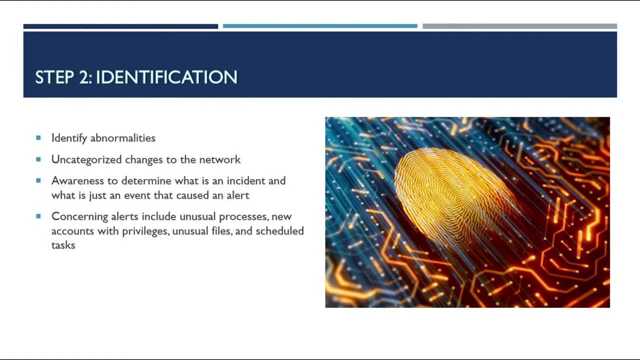 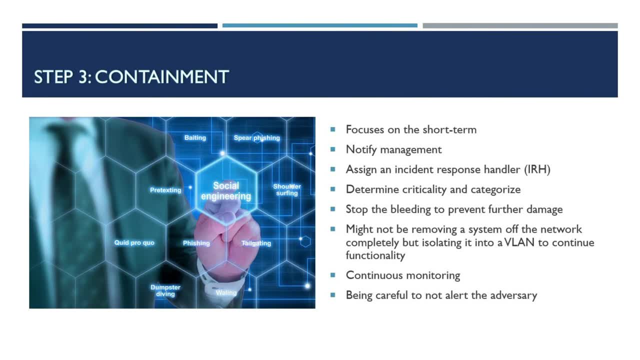 be unusual processes, new accounts with privileges, unusual files and scheduled tasks that are outside of the norm. Step three is containment. At this point, the focus is on the short term and you should begin alerting management. This is also where the incident response handler is assigned. 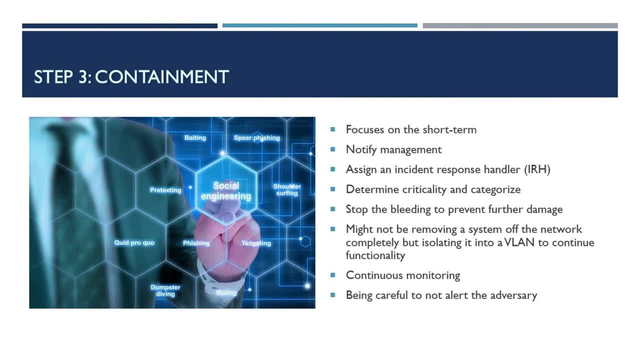 and starts the process. You must stop the bleeding and prevent any further damage and determine the criticality of the situation and categorize, while also containing, whatever is affected. Before taking a system completely off the network, it should be determined what might be going on. If a system is vital to a business operation, impulsively taking something offline. 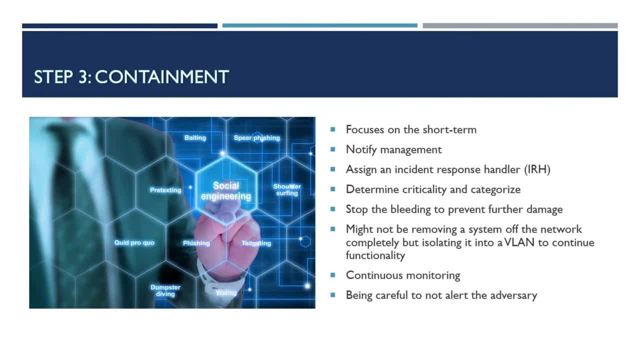 before understanding the event could have a more detrimental impact on the business. That's why containment might not be completely taking a system off the network, but it could mean isolating it in its own VLAN in order to monitor or cut it off from other systems. 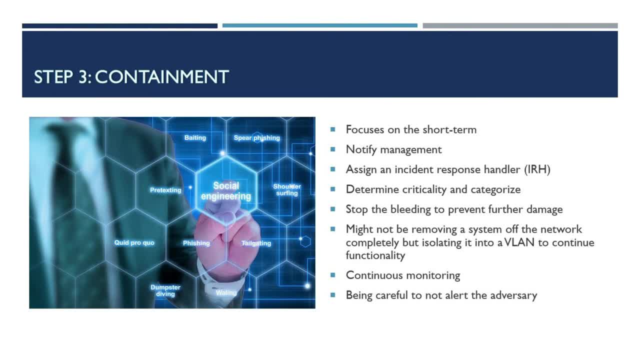 to prevent further infection. Another thing to keep in mind is that isolation, versus completely taking something offline, is that adversaries might be made aware that you know they're in the network and it might be better to monitor them. When you isolate it in a VLAN, the endpoint is still in the. 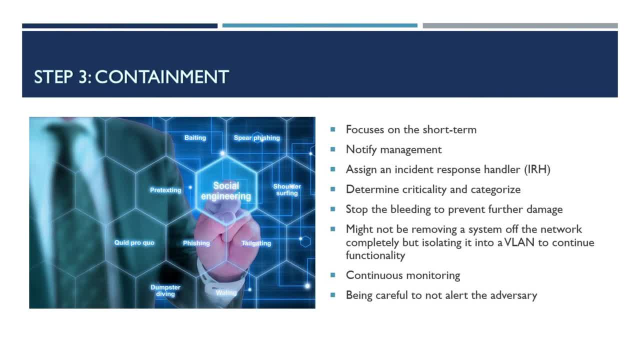 network, so it will still appear to be connecting to the C2, ultimately making the attackers believe everything is fine. This may not be an option if they've made it into an area with sensitive data or the attack surface could make eradication worse. 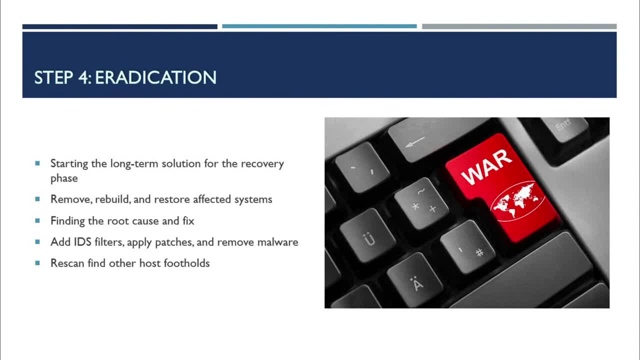 Step four: Eradication. This is the phase where you remove and begin restoring affected systems to start to work on a long-term solution to the problem. This could be figuring out the root cause and removing the malware from the systems by re-imaging. During this process, the network will be re-scanned. 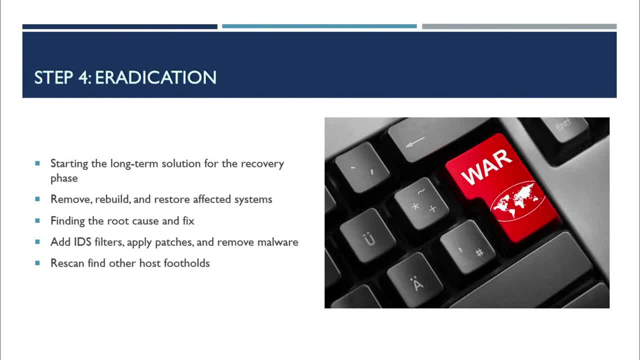 in order to find any potential footholds on other hosts. Depending on the scenario, someone may create scripts to locate and delete related artifacts and apply the necessary patches to prevent future exploitation. Overall, this is the beginning of the rebuilding and fixing the damage.